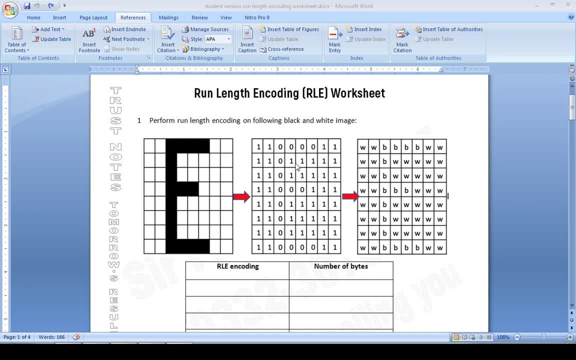 three, four and five number of whites, So we have written here five number of ones. This is how the binary conversion works. Then again, in the third row, we have got two number of whites, so we have written here two times one. Then we have got one black, so we have written here. 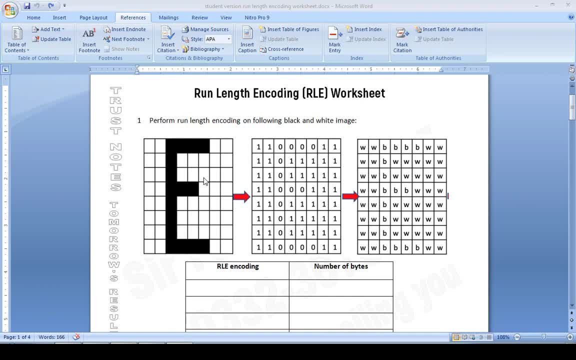 zero and then one, two, three, four and five. So we have got five number of ones. This is a binary representation. Now we apply run blended coding So it start with the first row. We have got two number of ones means we have got two number of whites, so we have replaced it by two. 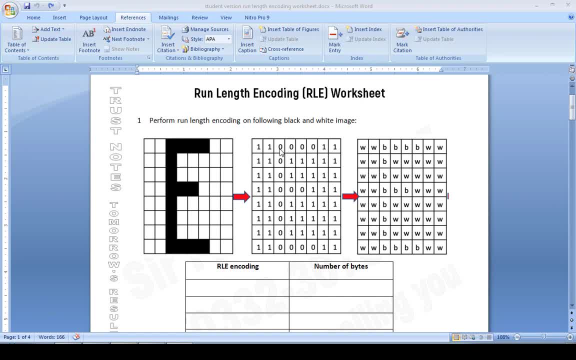 times W. Now let's interpret this black color. So one, two, three, four, four times zero. so we have written here four times B. Then we have got two number of ones which indicate white. so we have written here W. Same we will do in the next row. 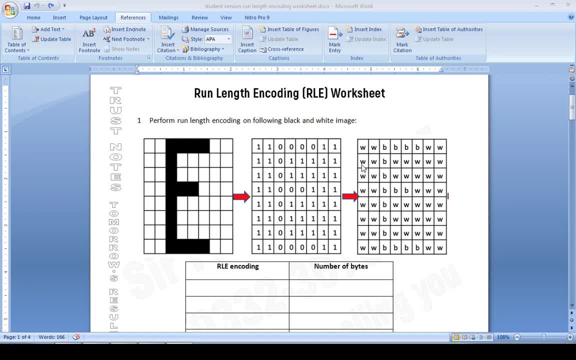 We have got two number of whites, so we have replaced one with the white W and one with the W again. Then we have got one black. then we placed one B, then one, two, three, four white. so we replaced the number one with the alphabet term which indicates white. 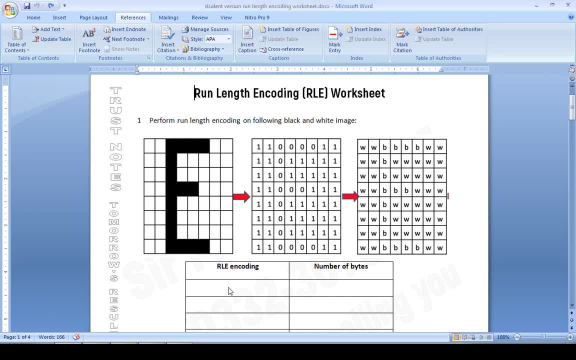 color. So this is pretty much interesting, but it is just keep getting better and better. Now, if we consider this portion of code, now we are applying further more run blended coding. So how do we compress the data? This is the compression time. So, row number one, we have got two number of W. 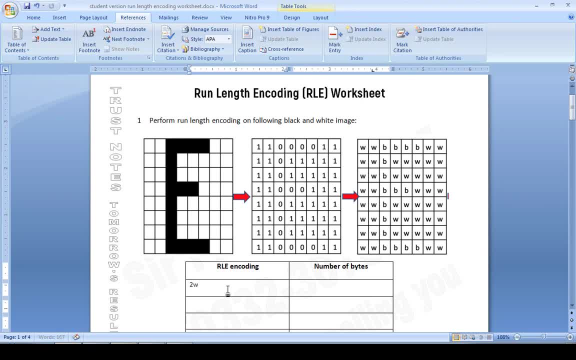 So we write in our table two W. Now I give some space for my understanding. Now we have got four number of white blacks, so I write for counting and a black color. Then we have got two number of whites again, So I write counting that we have. 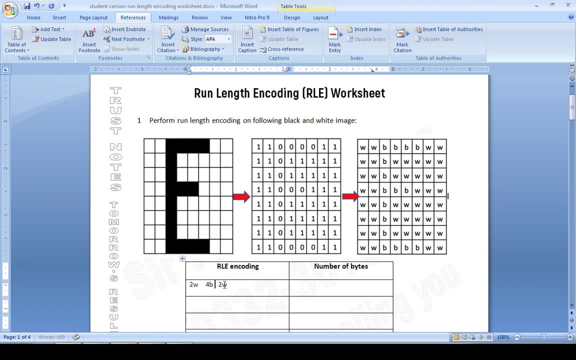 got two whites and I write W. so this is for the raw number one. so I write here: raw number one. okay, now next raw number two. let's interpret this raw. okay now, in the second raw, we have got again two number of whites, so I write two W. then we have got one black, so I write one B, then we. 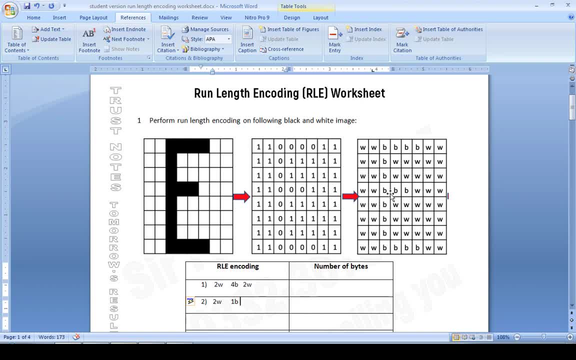 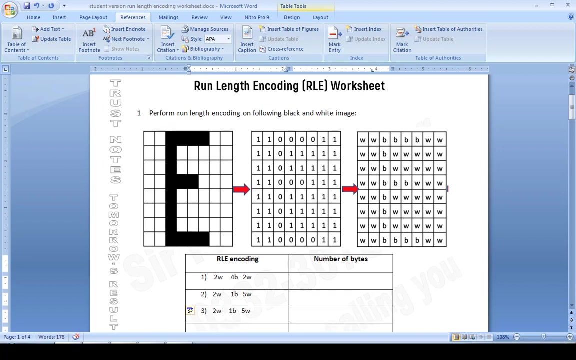 have got one, two, three, four and five. five number of whites. so I write five W. now repeat the same process again for the raw three, so raw number three. again two number of whites and one black and again five number of whites. now next draw number four: one, two, three and four. 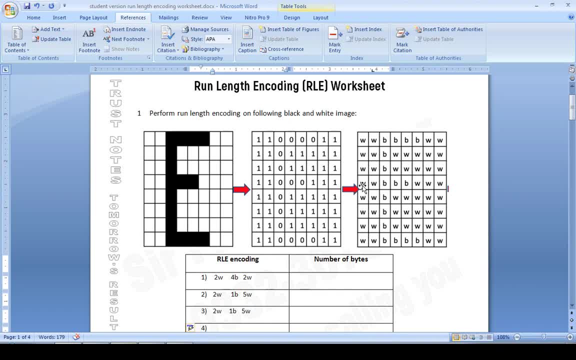 two, two, three and four. and two, two, three and four, and one, two, three and four. two number of whites and three number of black. two number of whites and three number of blacks. and then, okay, now next one, two, three, four. we have got three number of whites. 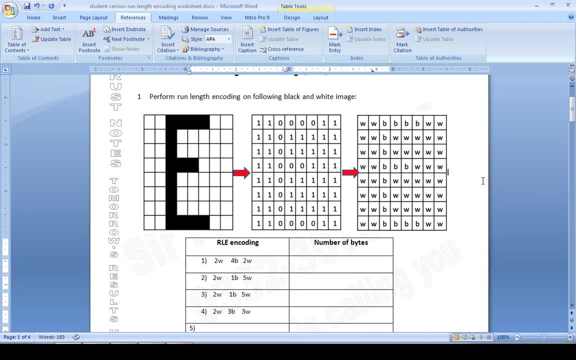 next same thing will be done with the row number five. okay, now let's start counting one, two, three, four and five. so we have got two number of whites and one number of black, and we have got one, two, three, four, five, five number of white colors. now raw number six. 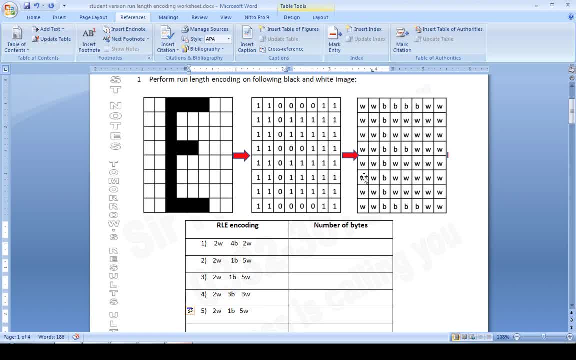 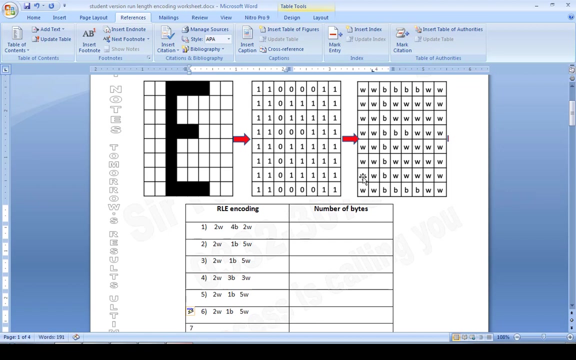 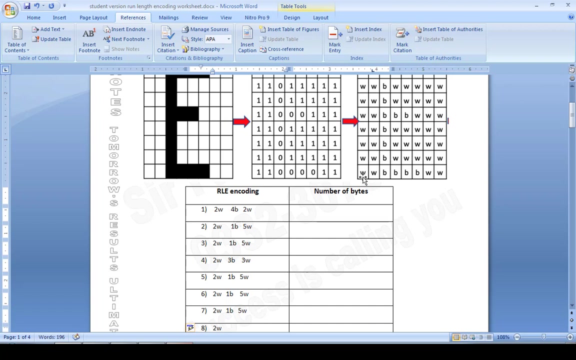 one, two, three, four, five and six. okay, raw number six: two whites, one black and five number of whites again. now raw number seven: two whites, one black and again we have got five number of whites. then row number eight, last row: two white, four black and two whites. 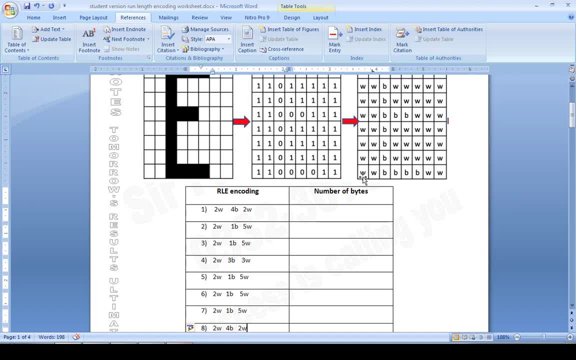 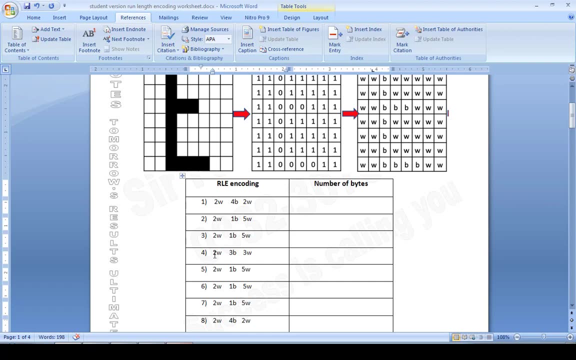 okay, i hope it is cleared. okay, let's just do a cross check that we have done correct or wrong. so let's start checking. two, four, eight, okay, all right, this is done, nicely, done right. all right now, it's done. now. next step is the is to find a total number of bytes, so let me 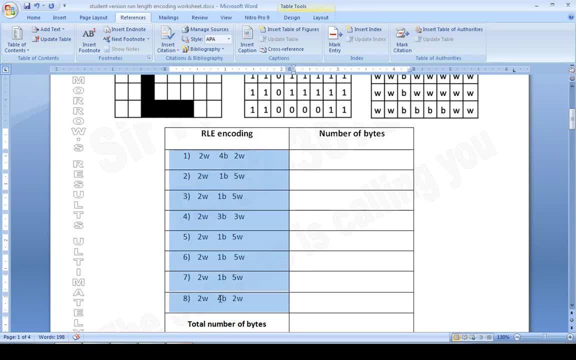 zoom it for you and let me do a little bit, a little bit bold, to increase the readability. so let's start counting for the raw number one. i, uh, i'm counting, okay, so one, two, three, four, five, six. so we have got six bytes here. okay, let me hold it for you two as well. 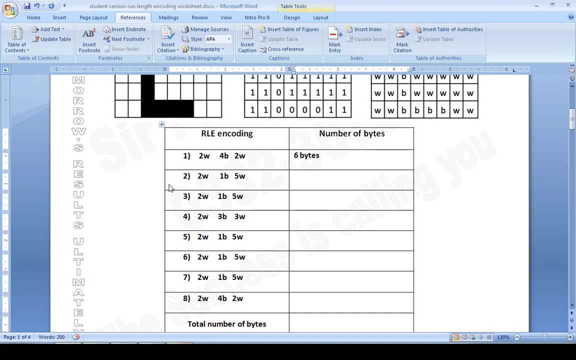 all right, so next row, number two. we have got- uh, let's start counting- one, two, three, four, five, six. we have got again six bytes. seems pretty much easy now next: one, two, three, four and five, six. what a coincidence. we have got another six bytes. next, again, start counting one, two, three, four, five, six. okay, no problem, so all of the bytes are somehow. 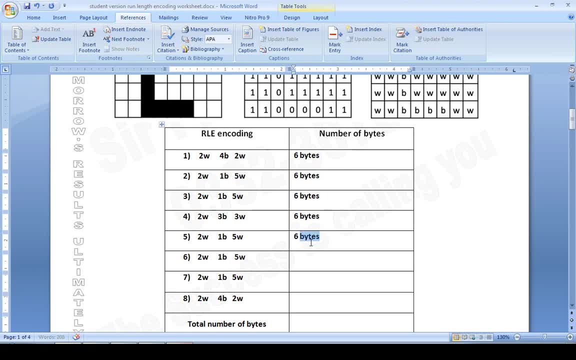 six. so if we just keep counting we get same number of six bytes. it is a coincident, it is not a fixed value. like you always get the six. five may be possible in raw number two you might get 10 bytes. or raw number three, you might get 15 bytes. raw number three, you might get. 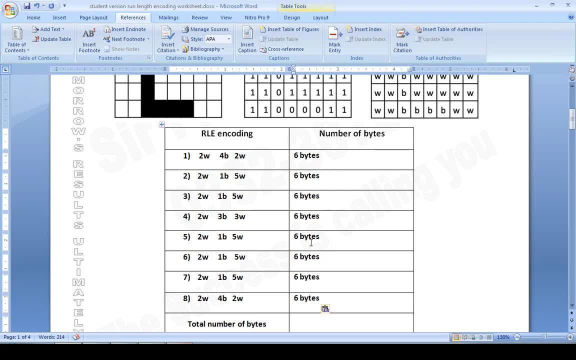 raw number four, you might get one byte or two bytes, or draw number nine may be possible. you might get 15 bytes. so this is not the fixed value that you always get the six bytes. this is basically a coincidence. so now let's start counting the total number of bytes: 6 plus 6, 12 plus 6: 18. 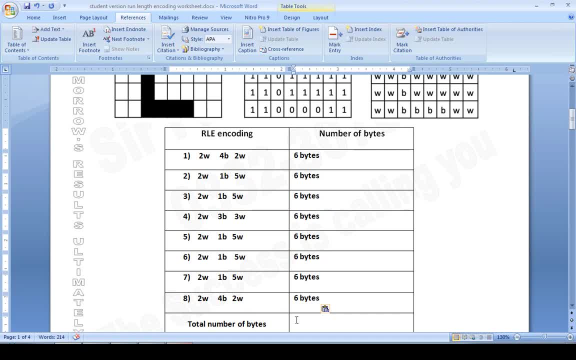 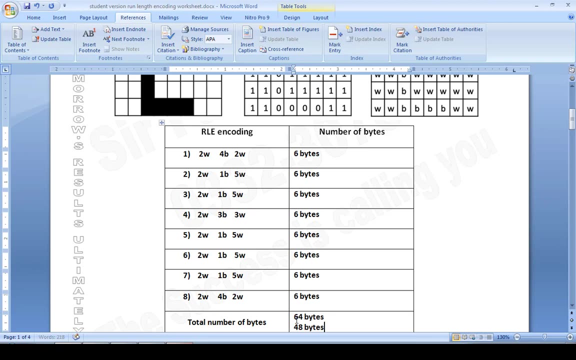 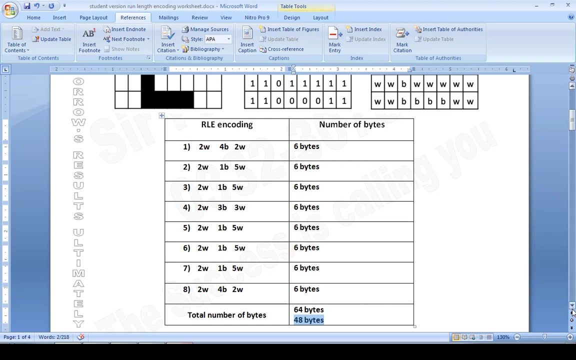 and so on. so when you count it so it becomes approximate 48 bytes. so the grid size is: if you talk about the grid size, it is of 8 by 8 means the grid size is 64 bytes. and how much our rather encoding compress the data and it allows, uh, only 48 bytes. so we are just consuming 48 bytes out of. 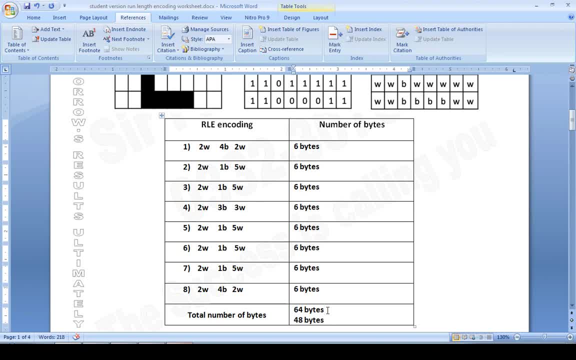 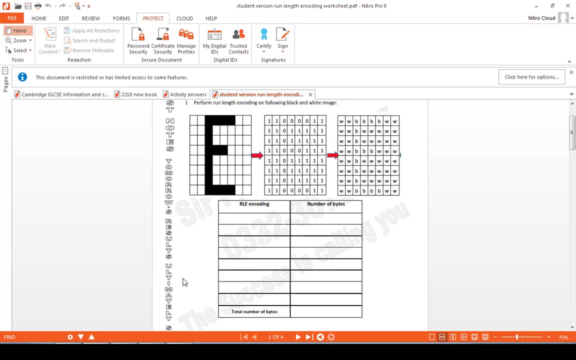 64 bytes, so pretty much storage has been saved. this is how we have to do. i hope you understood it and i am about to share the worksheet with you guys. okay, this is a worksheet that i have taken the images from the website and i just drew the table.